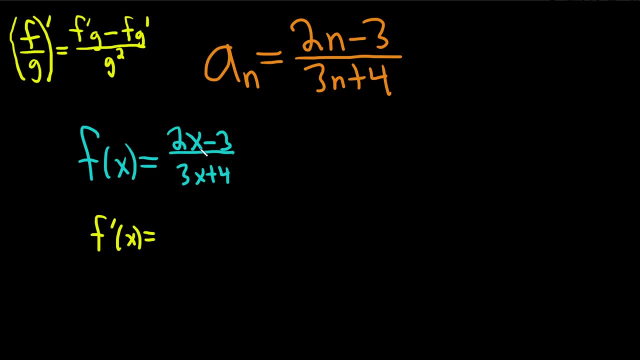 of x. so let's see: the derivative of the top is 2 times the bottom, so 3x plus 4 minus the top, So 2x minus 3 over 3x plus 4.. So 3x minus 3 times the derivative of the bottom, so 3.. And it's all over the bottom. 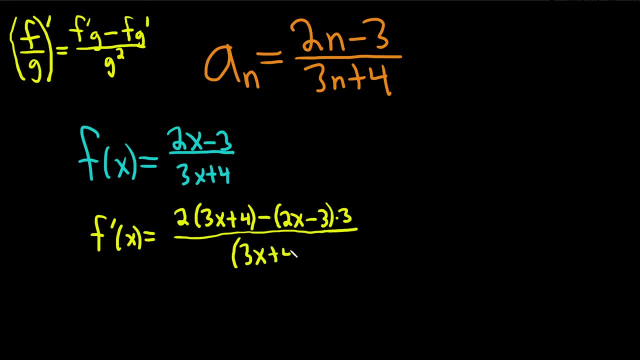 one and the whole thing is squared. And again, what are we doing? We're trying to see if the sequence is increasing or decreasing. so we're checking the first derivative. If it's positive, it's increasing, If it's negative, it's decreasing. Okay, let's clean this up. 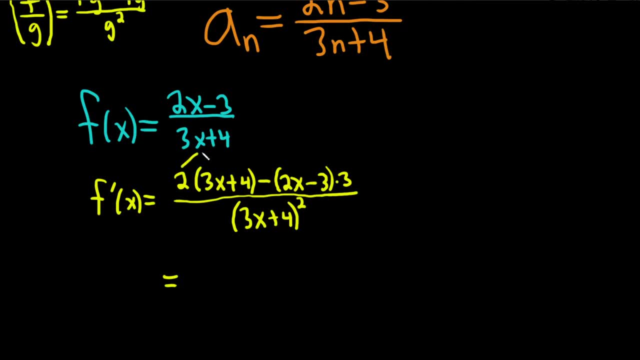 see what happens. Let's see this is equal to. let's see: 2 times 3x is 6x And 2 times 4 is 8.. I actually haven't done this problem yet, so this is kind of exciting: 3 times. 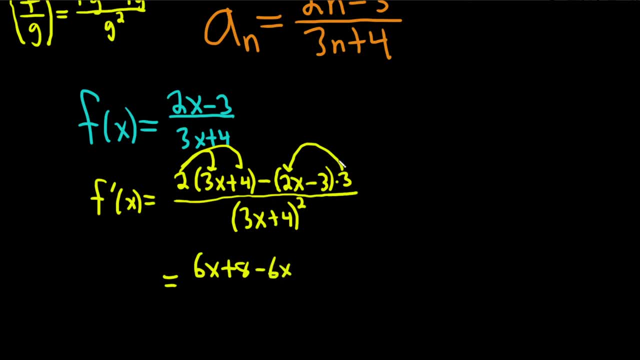 2x is negative 6x. Okay, oh, look, it's going to cancel. And then, oh, we've got to be careful here. Look, there's two negative signs, so it's a plus 9.. Oh, this is cool, This is fun. 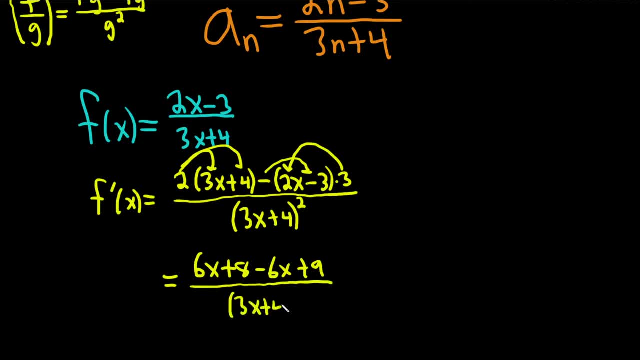 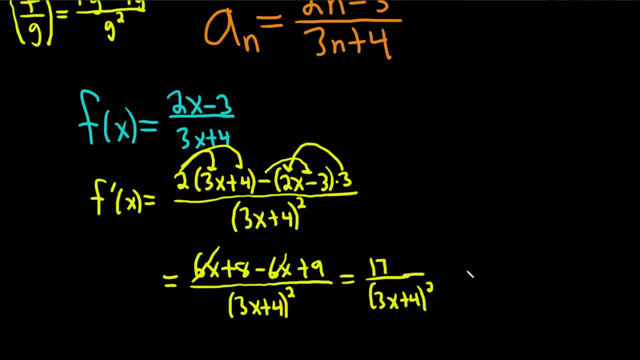 So you have 17 over 3x plus 4.. So you have 17 over 3x plus 4.. And that's squared. This is always less than 0.. Sorry, greater than 0. This is always greater than 0.. 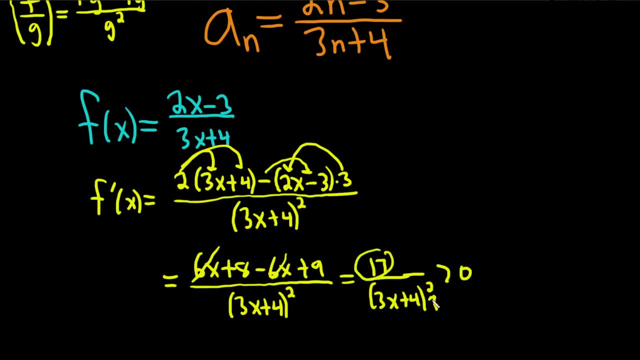 It's positive, right, This is positive. This is positive because it's squared. It's always going to be positive, for, let's just say, x greater than or equal to 1.. And I'm saying that because we want n to be greater than or equal to 1.. 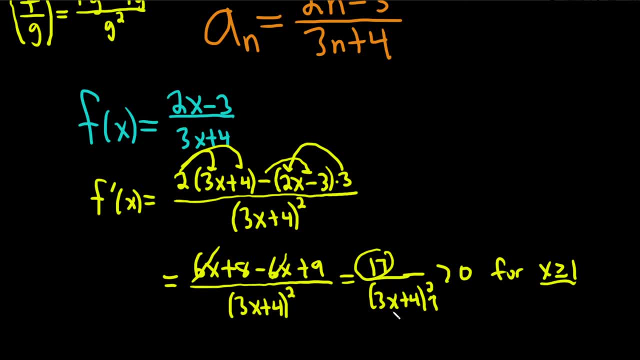 Obviously here. this might be well. it might be undefined if x is a certain value, but that value is not going to be here, right? The only time it's going to be here is if x is greater than or equal to 1..